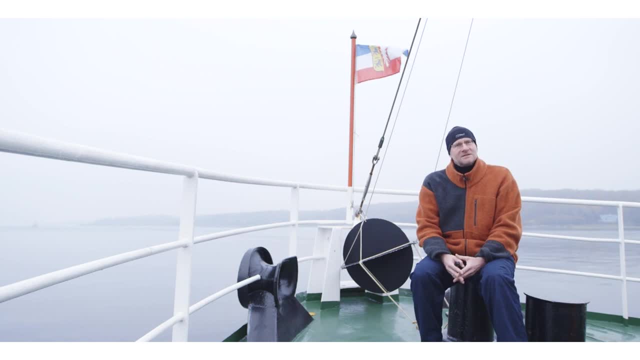 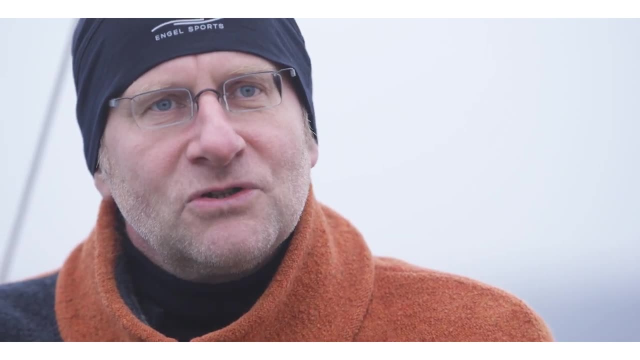 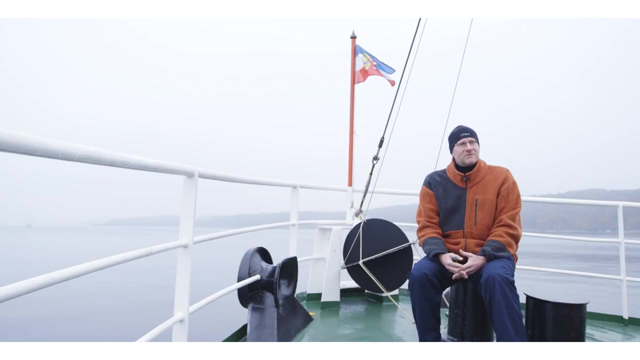 that previously has eaten a fox. So this is how marine systems work, very differently from land. If you look at a bucket or a bottle of ocean water, usually that's very transparent and you ask yourself: so what actually? where does life come from? that eventually will lead. to populations of fish that can be harvested. And actually people were asking that for quite a long time, way into past the medieval times, And it was only in 1887 that Victor Hansen took a plankton net. that's a net with very fine meshes, went out, sift through ocean. 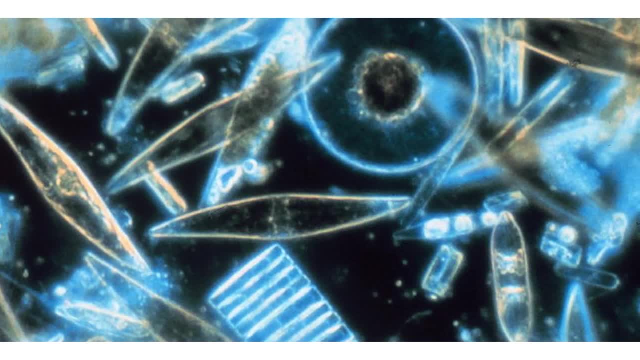 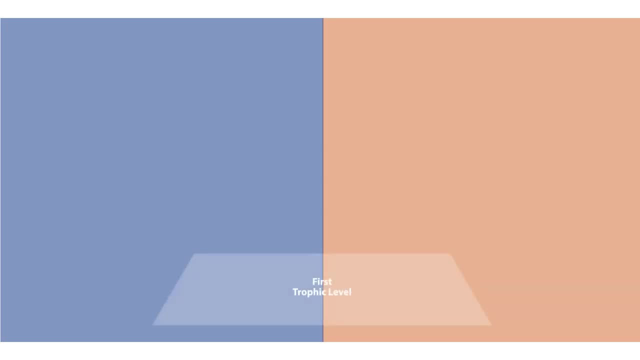 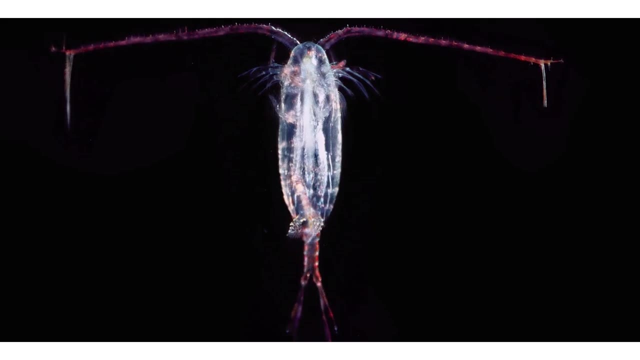 waters and, with the aid of a microscope, found tiny organisms, tiny plants that are actually at the base of the food webs And, through the process of photosynthesis, as we know it, from land they build up organic matter that can then be consumed by secondary consumers. 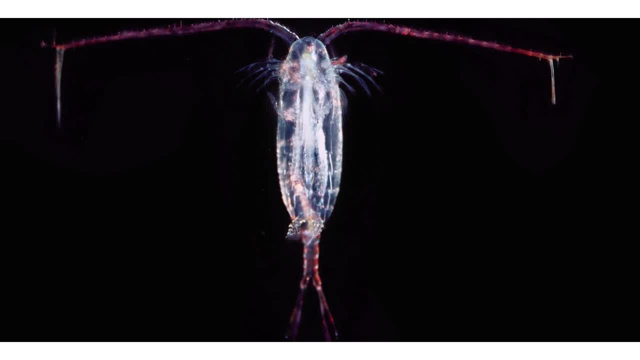 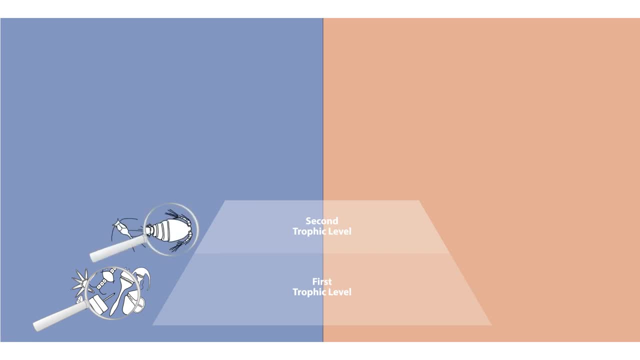 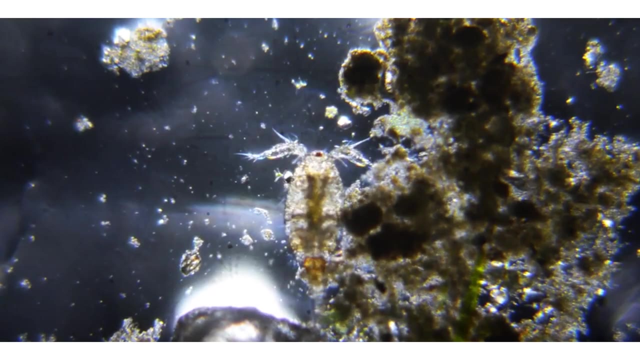 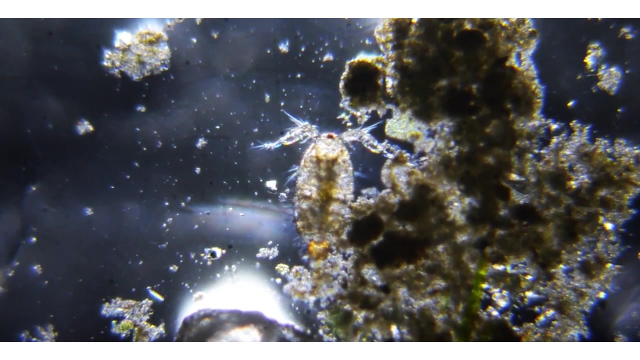 which are, if you will, the cows of the sea, tiny crustaceans called copepods. So since the plants with which the food web starts are very small, also the first consumers have to be quite small. And then those tiny crustaceans, and also larvae of worms and mussels that also have their 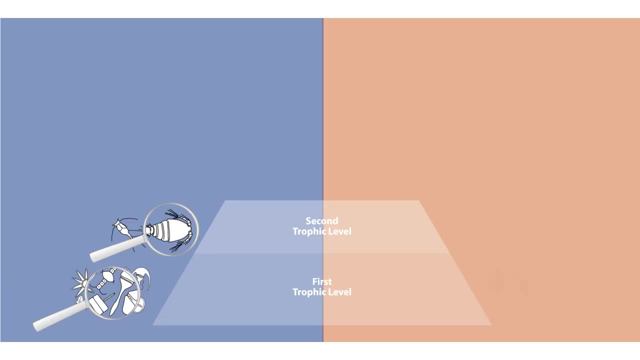 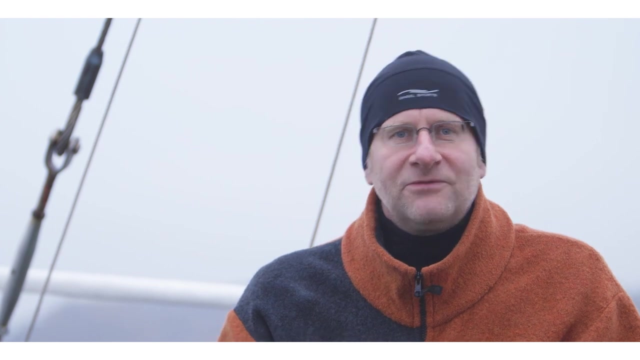 larvae in the plankton, feeding on phytoplankton. they are then consumed by still relatively tiny fish. so either juvenile fish or small anchovy, small pelagic fish. So we have already now three steps in a typical open ocean marine food chain that would lead to still a small. 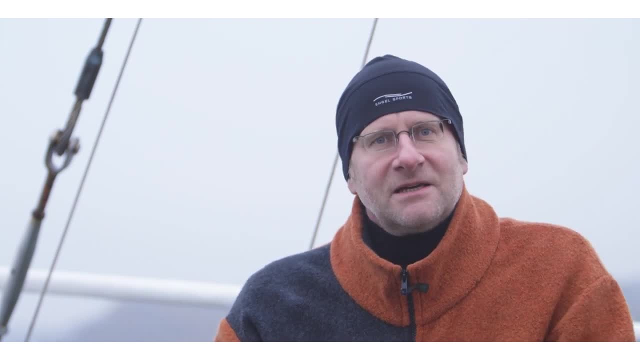 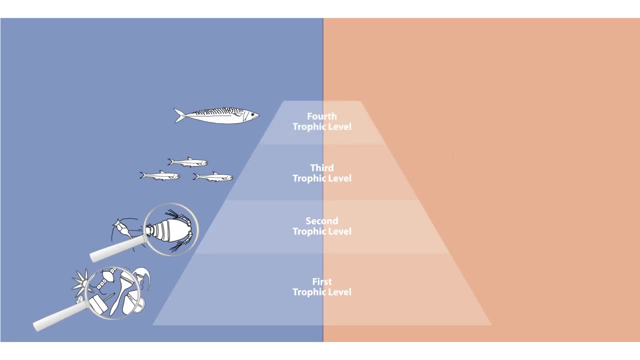 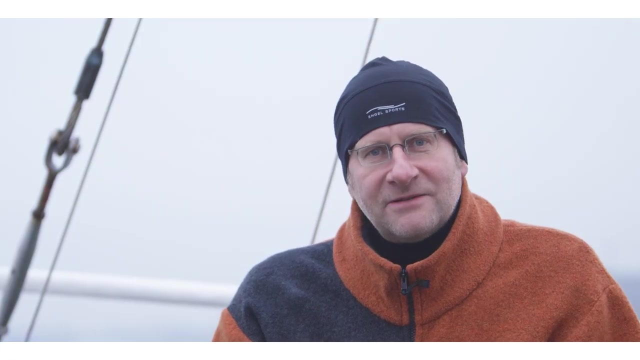 fish that we didn't yet want to put on our plate, Meaning that open ocean food webs usually take several steps, up to five or six steps, to end then in a big tuna or in a large shark. So why is this important? So why is that very significant for understanding marine productivity? 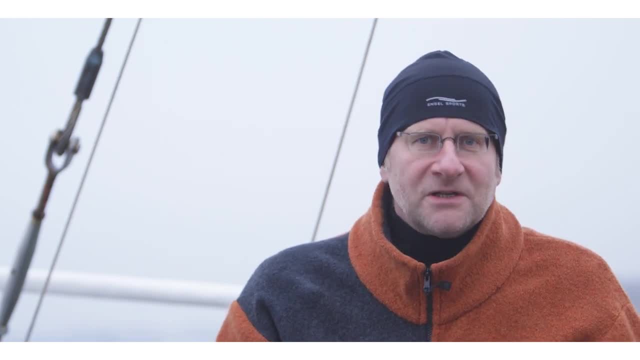 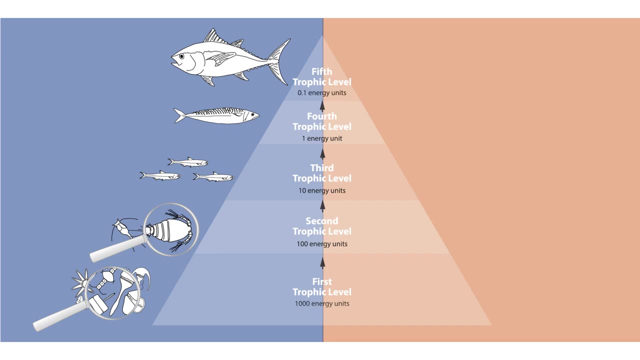 in general. Well, in each conversion, when one organism eats another one, about 90% of the biomass gets lost simply by respiration, by the maintenance metabolism of the organisms, and only 10% of the matter gets transferred to the next trophic level. And that means, if we eat a 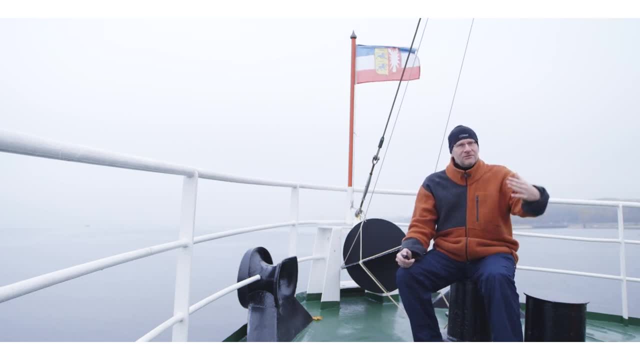 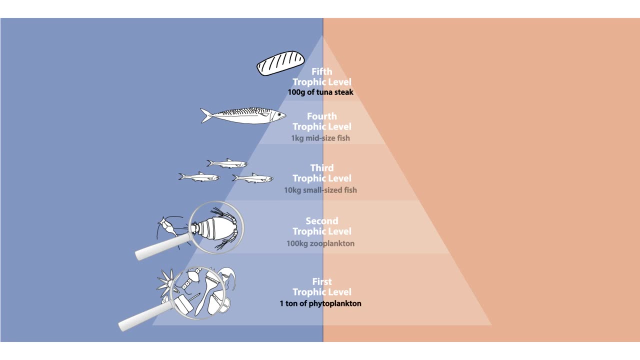 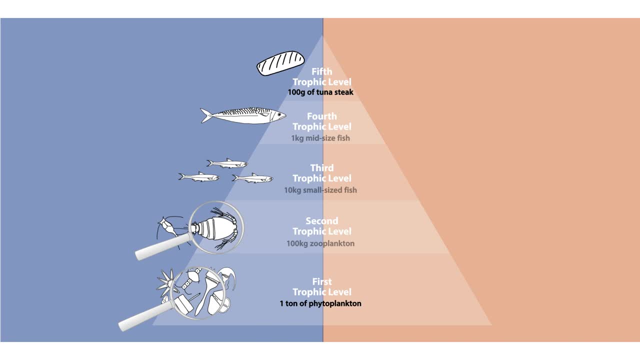 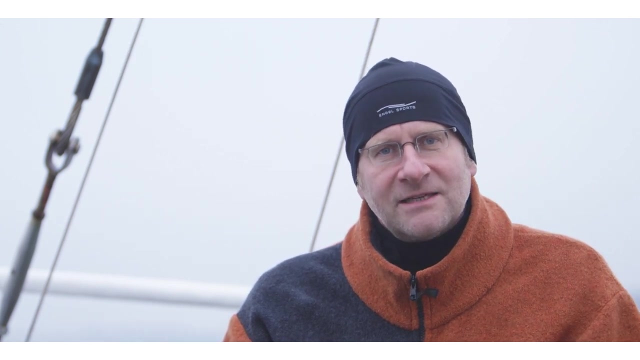 we need to build up one ton of phytoplankton biomass to sustain this 100 gram steak of tuna. And now you can hopefully see the significance. It means that, although oceans cover very vast areas and you may think that fish populations cannot, 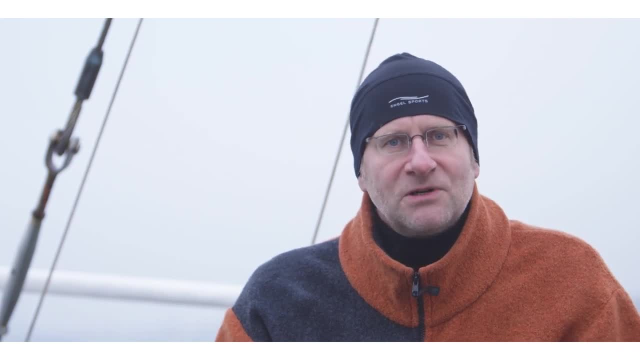 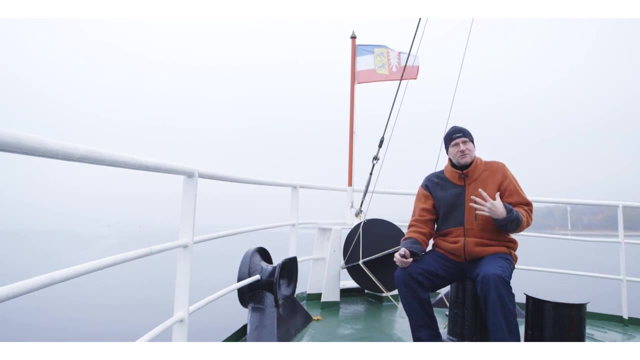 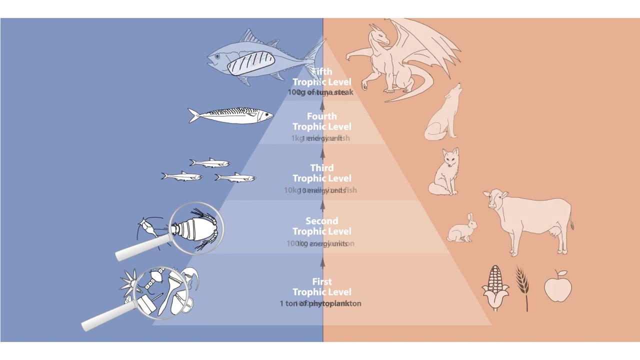 really be over-exploited. this is very much the case because the amount of biomass that goes into a fish population is very much reduced by the very long way through a relatively long food chain, And that's again very different to land where we can directly eat cattle. 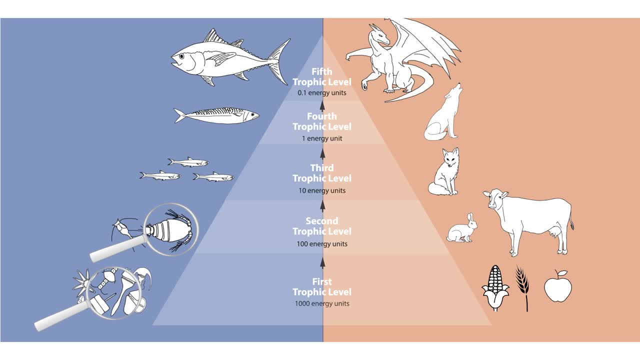 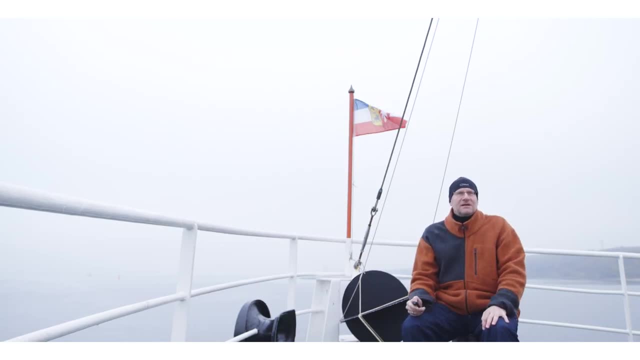 That's the first consumer directly eating on the primary producers, So having four trophic steps less than our tuna. So, to give you another example, if you put a mackerel on your plate, this would correspond to on land, on eating a. 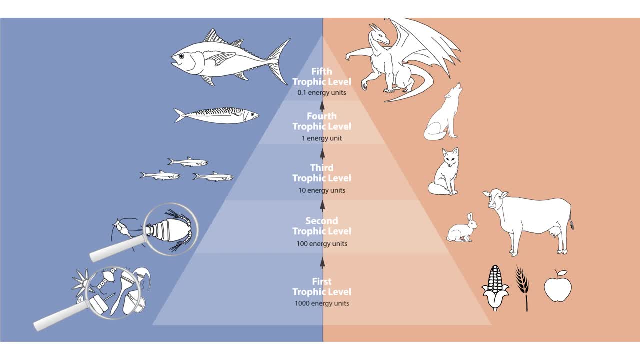 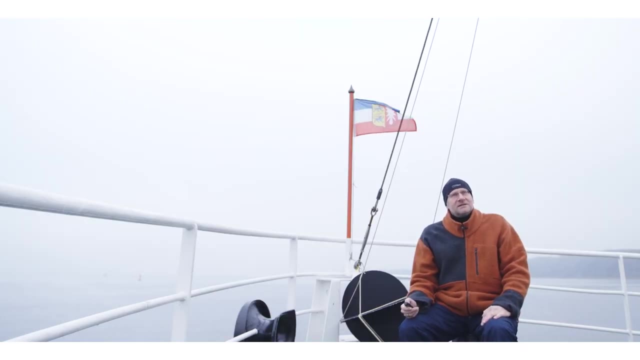 wolf, who has entirely fed on foxes, because a mackerel is already the fourth trophic level, And so we would be actually the eaters of wolf eaters, and so would be the tuna, And now you also understand why. the largest animals among the fishes and among the mammals 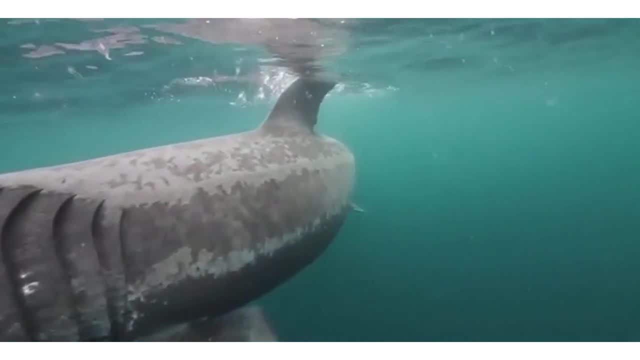 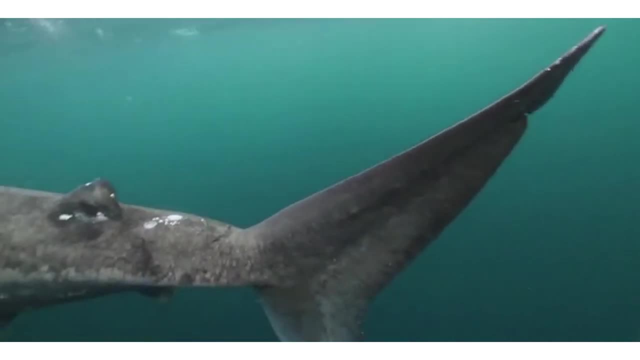 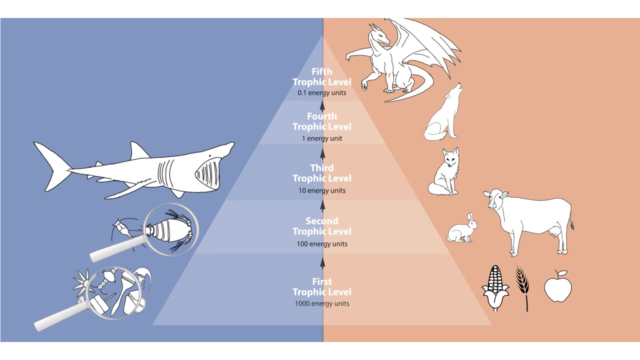 are filter-feeders That, by means of their filtering organs, either the baleen with the whales, or gill arches that are modified with a very large basket shark, go directly for the zooplankton for the first consumers, they themselves then being the second consumer. This is because 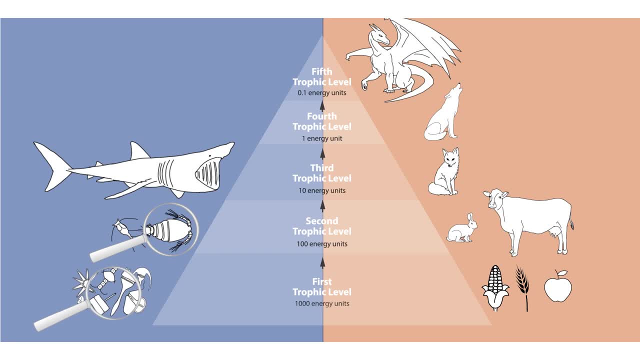 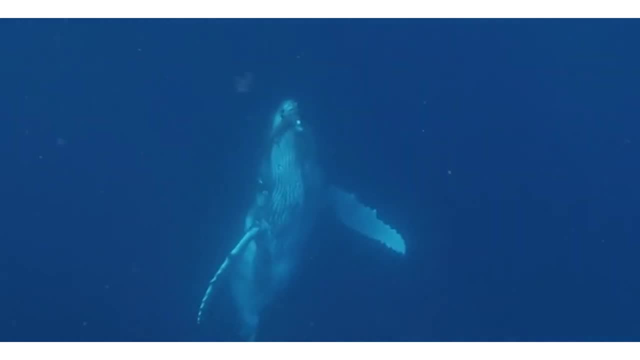 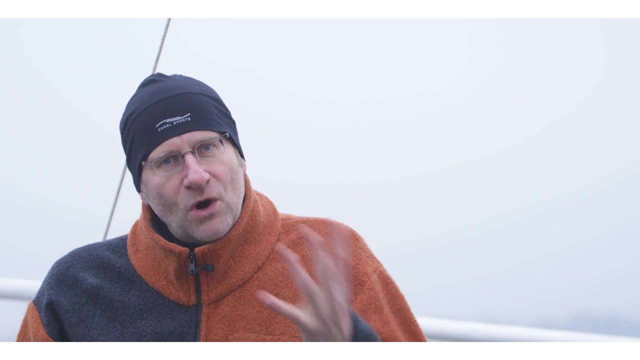 they spare all the upper steps of the food chain of the trophic levels and this way they can feed on much more biomass It's available and this is the only way how they can maintain their very large biomass. We now come from the open ocean to more coastal systems. Coastal marine systems are generally 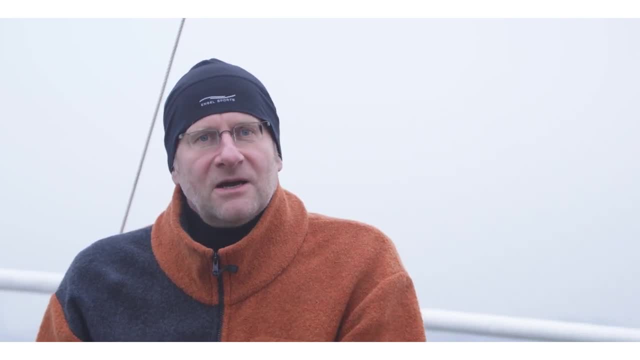 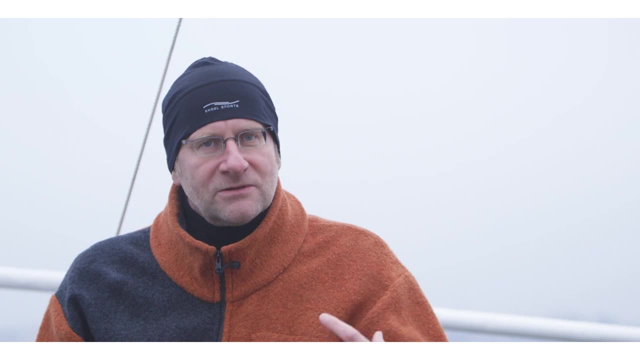 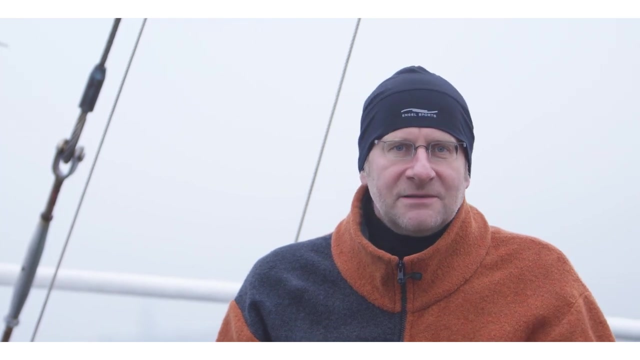 much more productive than open ocean systems. One reason is that we have a three-fold input into the food chain. It's not just the plankton that is also there, but we also have, in addition, plants that grow either on rock, like algae, or on sediments, like sea grasses, And then we have tiny unicellular algae that themselves 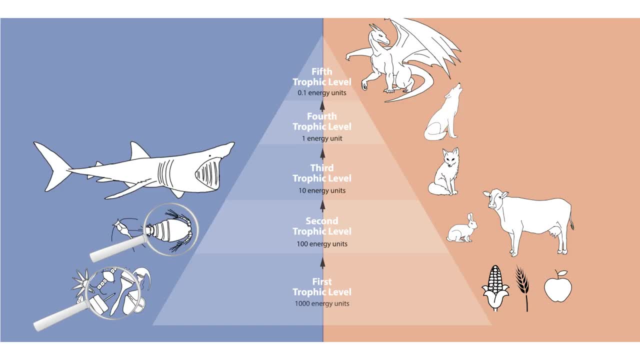 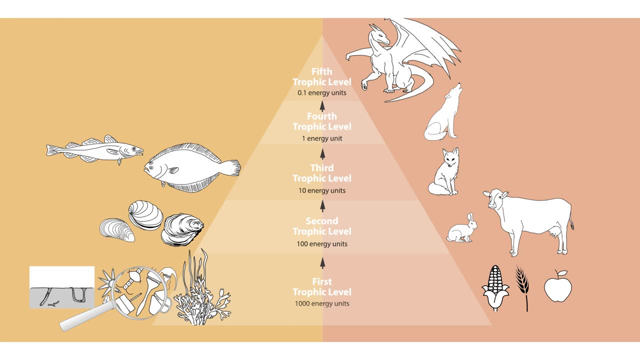 grow on the sediment surface or on the larger plants themselves, And also we can have very short food chains. The plant material gets degraded into detritus And, like earthworms, worms in coastal sediments- they directly eat on the primary productivity. 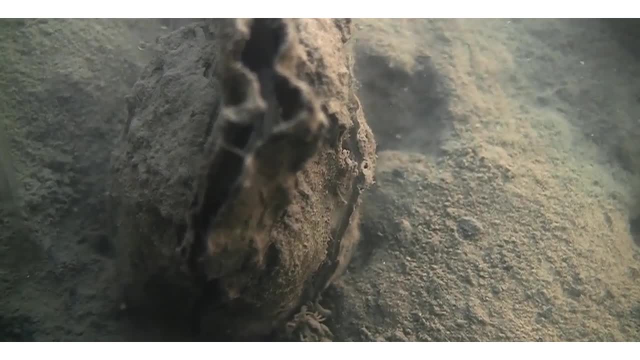 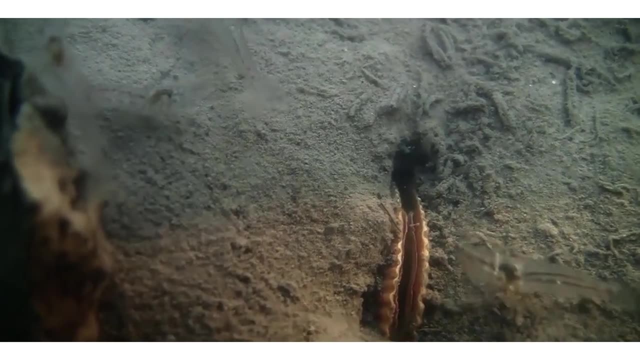 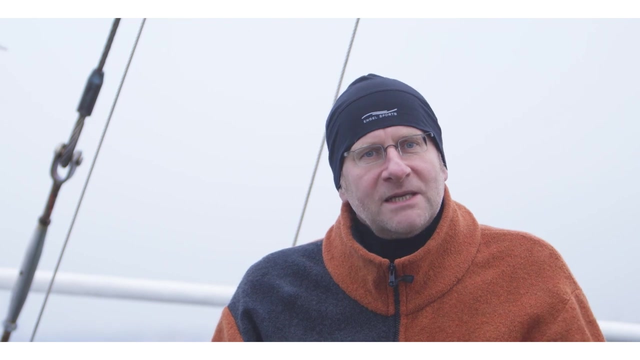 and also bivalves filter directly, the plankton, And then we have the bro碴 and these birds that can convert to or inject some vectors in various ways. so that can be a really interesting way in which the fish will be caught up. 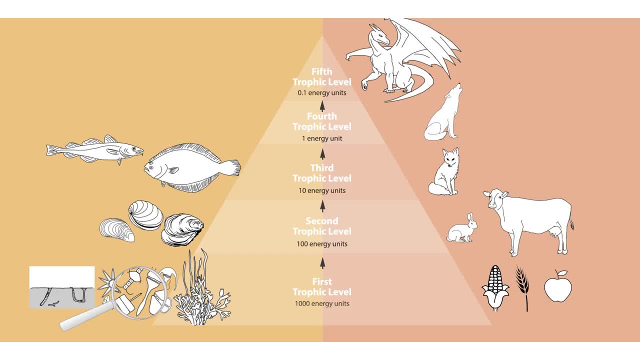 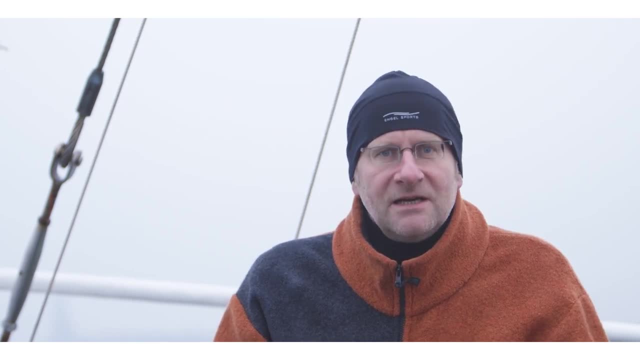 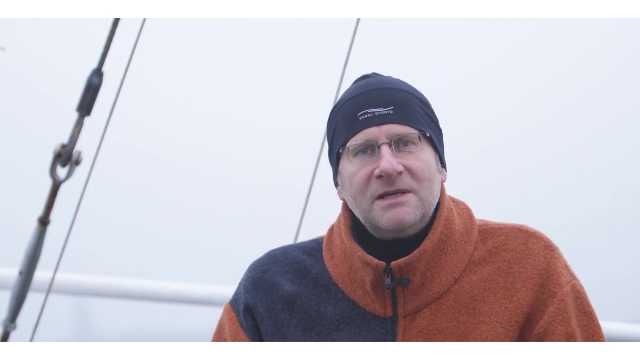 And then we have fruit systems that are AE Beef- Cor謝謝 for thinking they are thekatis br attorney too. And then this we have here. we have three retention groups. There is theulturist, commonly called the can only enter 150 to 200 meters to sustain photosynthesis. 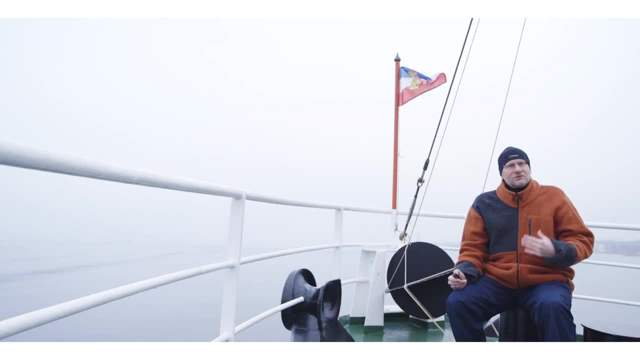 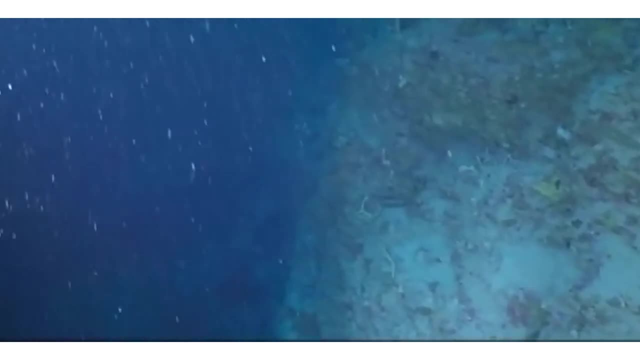 That means that most of the ocean that's several kilometers deep, so it relies on the production of the upper sundered layer And so dead particles that are sinking down from the upper sundered layer, be it dead phytoplankton. 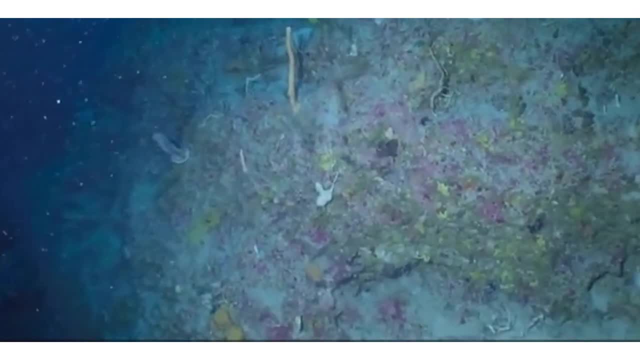 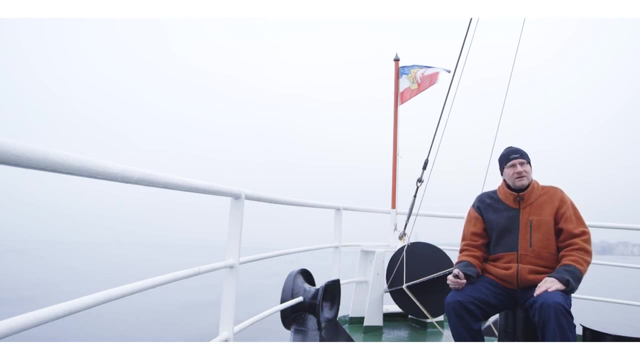 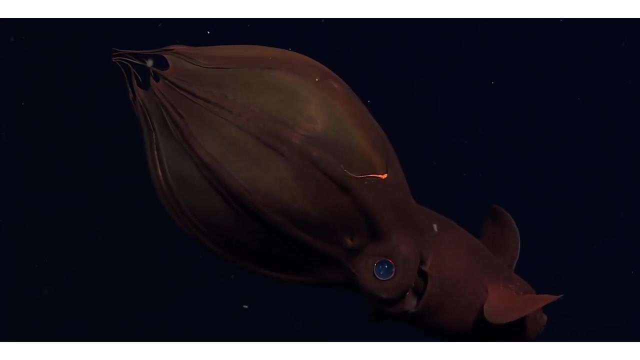 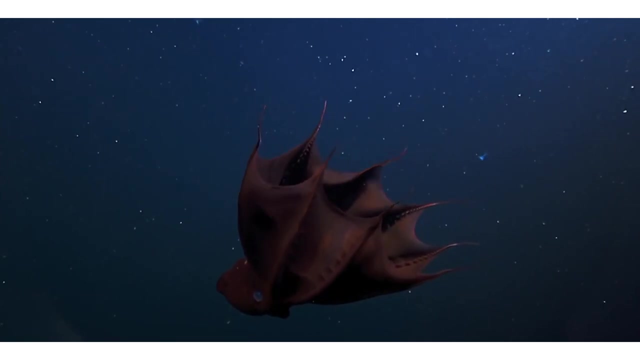 or the feces from other organisms that have fed each other, sinks the long way down to the deep sea bottom, And on that way there are specialized organisms like the vampire squid that are specialized on going after that sinking menu that has still some calories to digest. 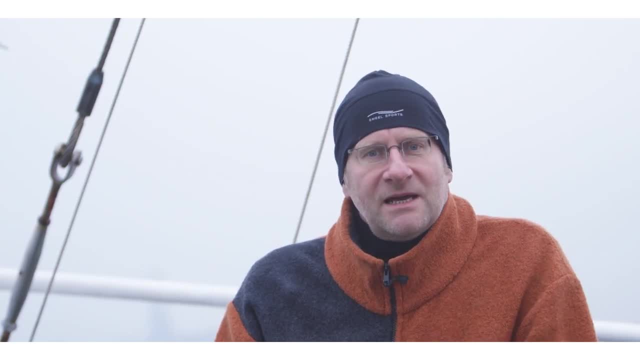 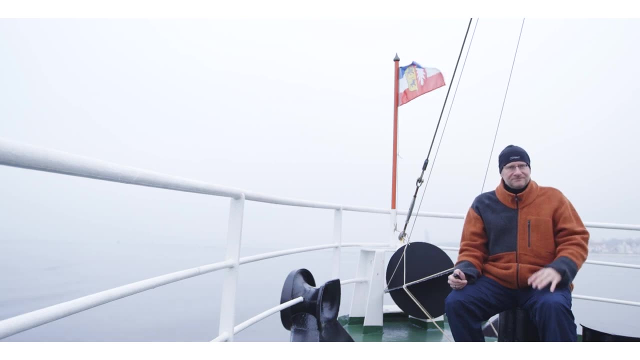 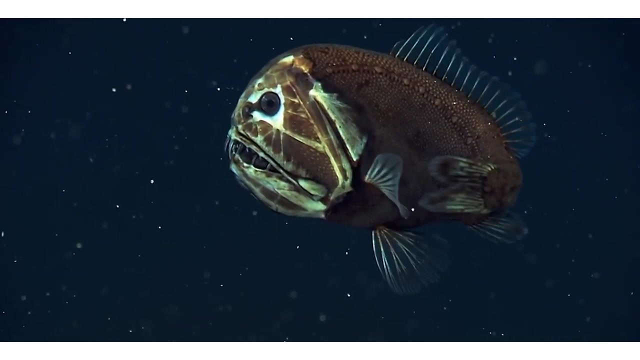 And once this rain is down at the deep sea bottom, it has gone down to 1% or less of the digestible biomass that has been there in the sunlit upper surface. This then again means that many of the deep sea organisms have to adapt to extreme food shortage. There are very low population densities and many other adaptations, like longevity and very slow growth, that these deep sea organisms need to survive. So I hope in this chapter you have learned some basic structural features of marine food webs that are very different. I hope you have learned some basic structural features.